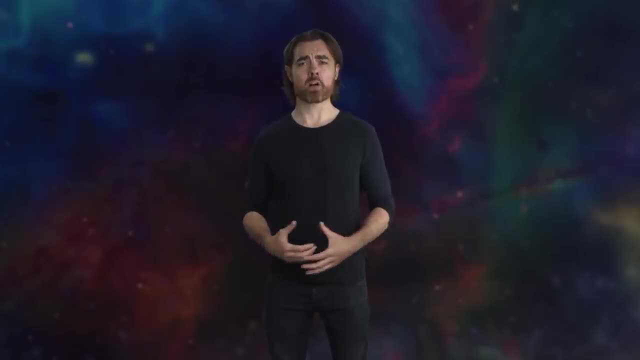 since that golden era of physics, we've been trying to reconcile the two, without success. But today, on Space Time, I'm going to begin our discussion of the great quest for this union, The quest for a theory of quantum gravity And for a theory of everything. 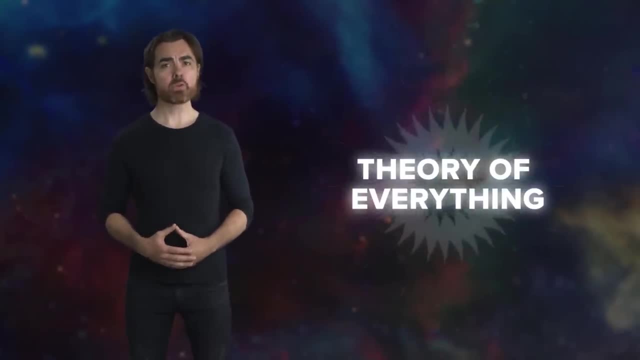 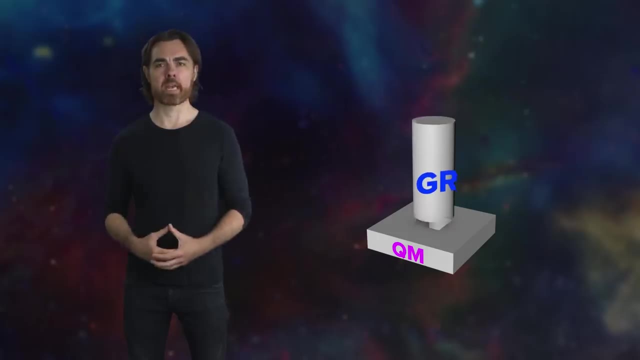 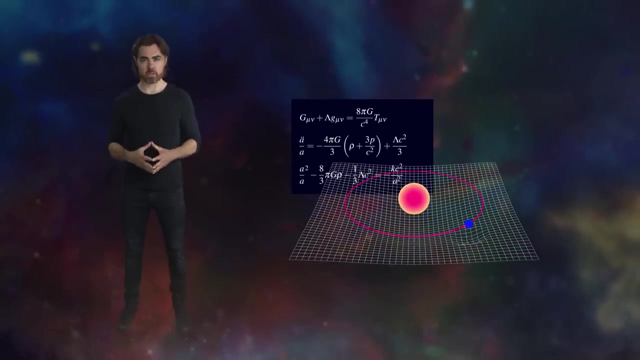 This is a big topic, So in this episode I want to give you the motivation. What exactly are the conflicts between general relativity, or GR, and quantum mechanics? I'll save the solutions for future episodes. Let's start with summaries. General relativity- GR- is Einstein's great theory of gravity. 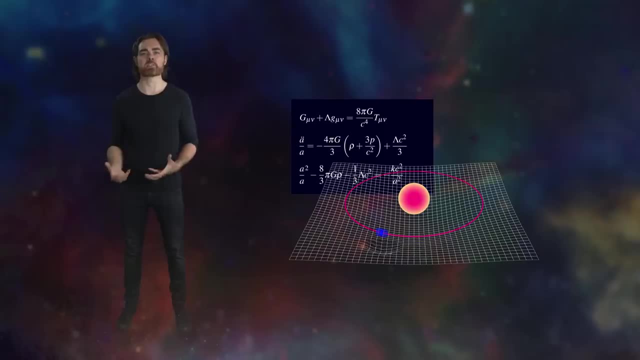 In it. the presence of mass and energy warp. the fabric of space and time And the motion of objects is thereby altered. This results in the effect we perceive as gravity. General relativity incorporates the earlier special relativity, which describes how our perceptions of space and time also depend on motion, Unlike the earlier ideas of Isaac Newton, in which 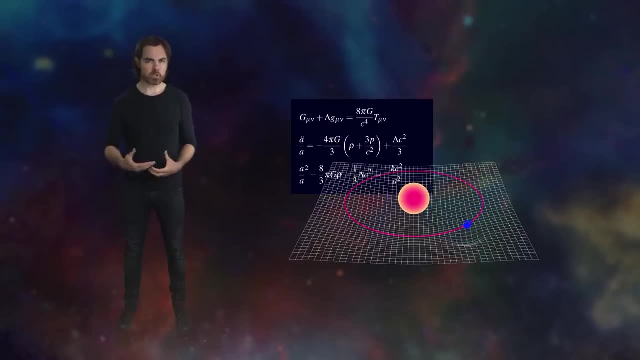 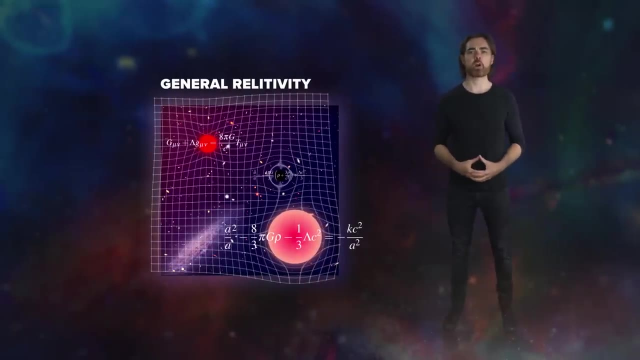 space and time are treated as separate and universal. special and general relativity blend them together into a combined mutable space-time, Where general relativity describes the universe, of the living world and the time in which it's crossed over is. 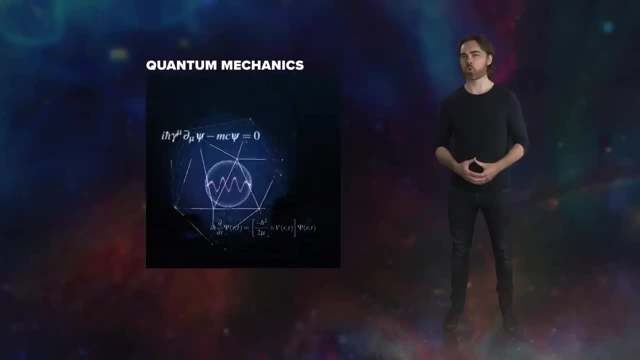 1. South-East Europe has taken a step forward in a national or secular, Paganistic fine arts. large and the massive. quantum mechanics talks about the subatomic world. It describes particles as waves of infinite possibility whose observed properties are intrinsically uncertain. 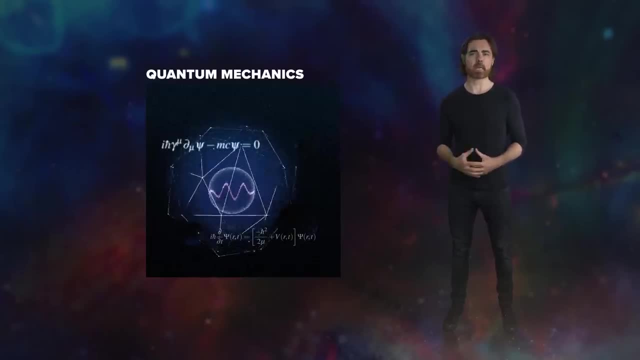 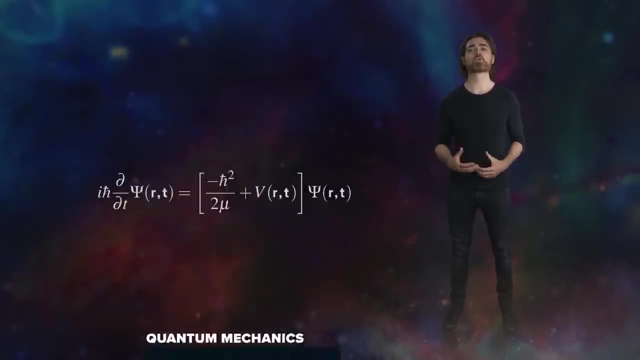 Our experience of the universe appears to be plucked from this landscape of possibilities in strange but mathematically predictable ways. That math started with the Schrodinger equation, which tracks these probability waves through space and time. But the Schrodinger equation treats space and time. 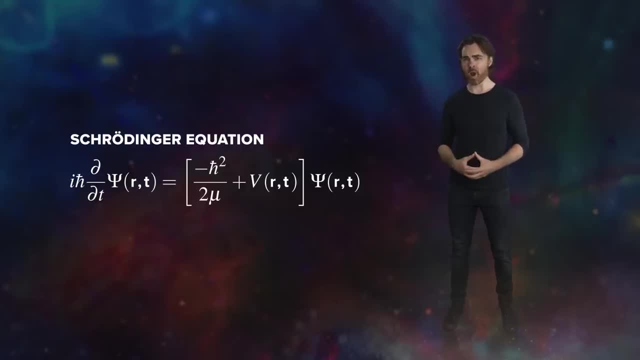 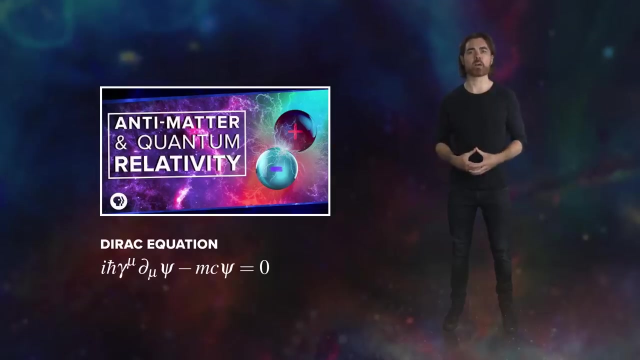 as fundamentally separate in the old-fashioned Newtonian way. So clearly there's a problem. We already talked about how Paul Dirac fixed part of the problem with a relativistic wave equation for the electron. Nowadays, modern quantum field theories fully incorporate the melding of space and time predicted. 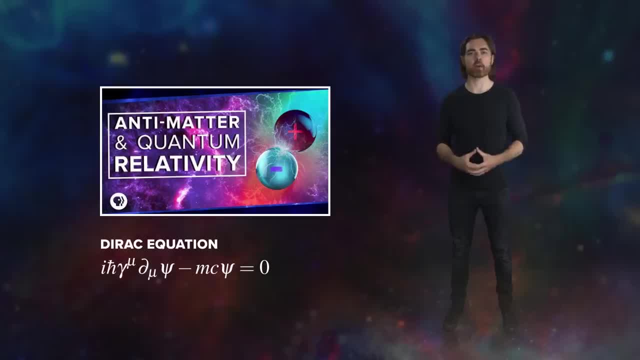 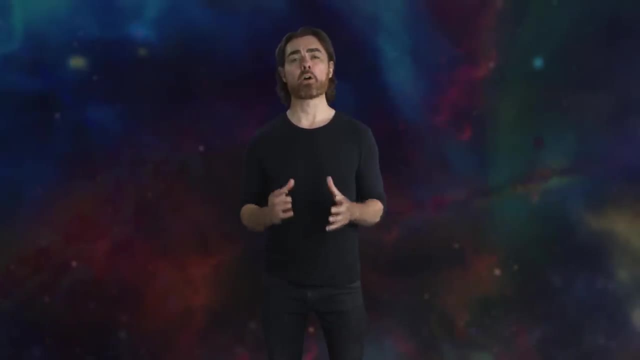 by special relativity, And yet they still don't directly incorporate the warping of space and time predicted by general relativity. This causes issues, Some mild and fixable, others catastrophic. Starting with the mild, we have the black hole information. 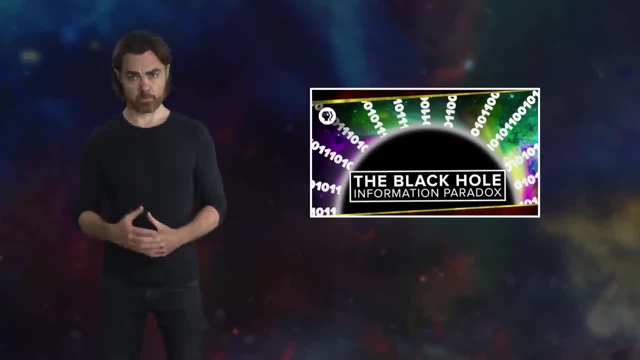 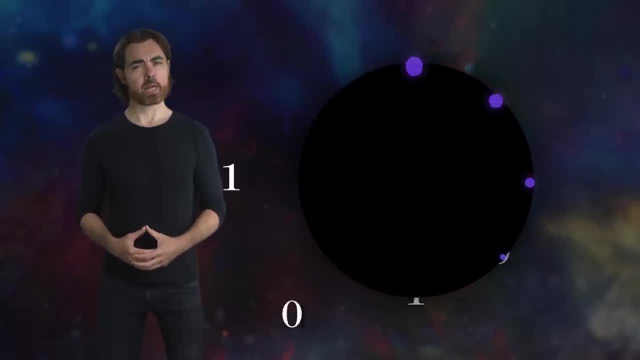 paradox. We've gone on about that at length. The black holes of pure general relativity swallow information in a way that can remove it completely from the universe, especially when those black holes evaporate via Hawking radiation. That's a big conflict with quantum theory. 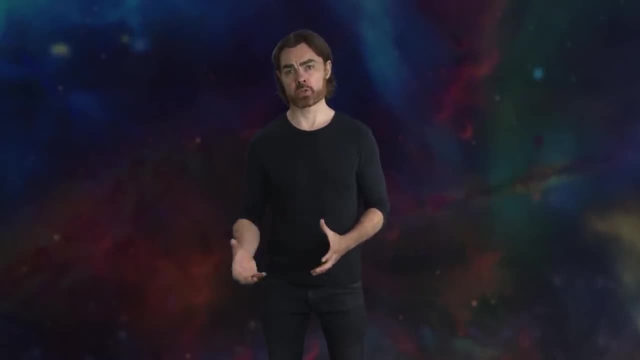 right there, which tells us that quantum information should never be destroyed. But that same Hawking radiation offers part of the solution to the information paradox. Following the work of Hawking, Jacob Bekenstein, Gerard Uthoff and others, it has become clear that information 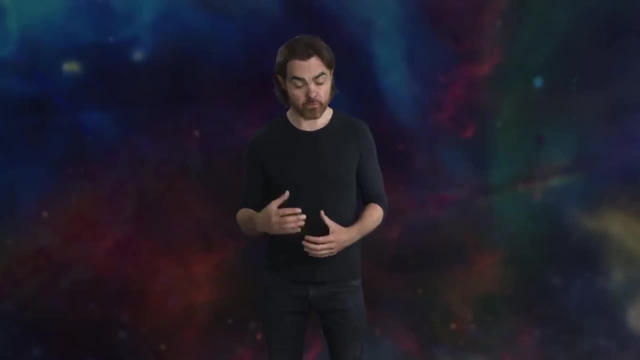 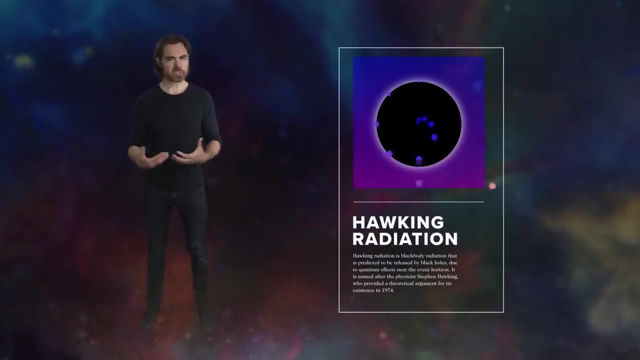 swallowed by black holes can be radiated back out into the universe via their Hawking radiation. In a sense, both the source and the solution to the information paradox came from the discovery of Hawking radiation. Hawking actually derived the latter by finding a way to unite. 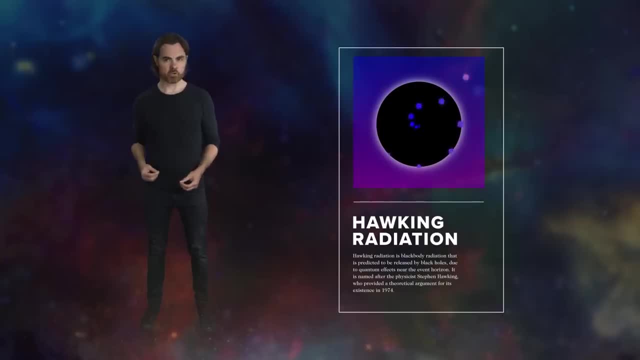 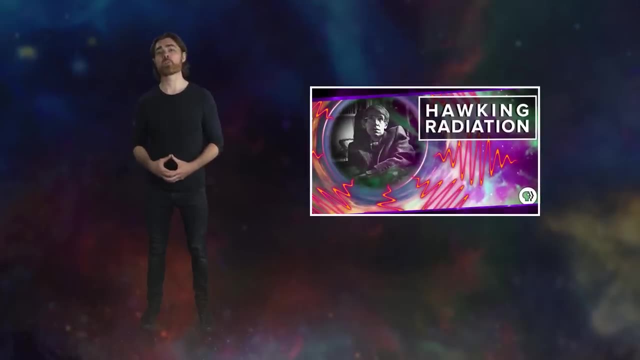 general relativity And in fact it's very possible to shoo-horn the curve geometry of general relativity into the way quantum field theory deals with space and time. But that approach completely fails when you have strong gravitational effects on the smaller scales of space and time. 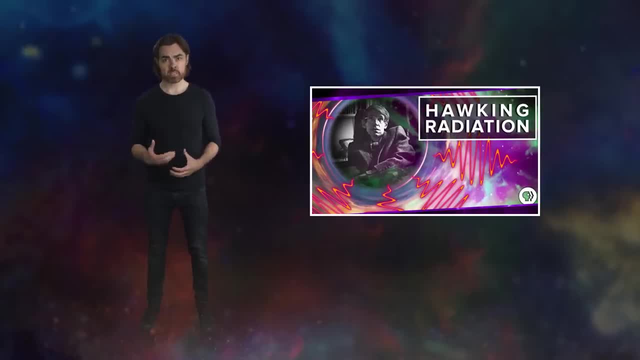 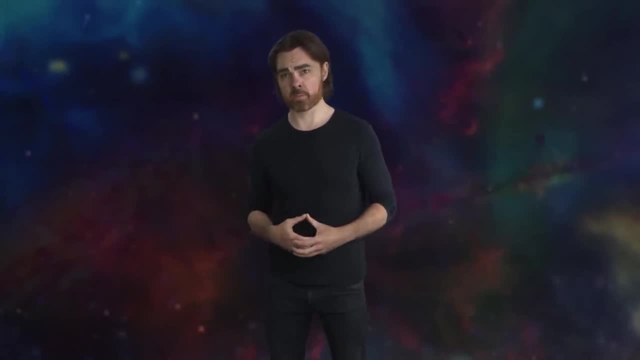 like the central singularity of the black hole or at the end of the black hole. So the theory of the black hole is a little bit different than the theory of the universe. It's a little bit different than the theory of the universe. But it's a little bit different than the theory of the universe. 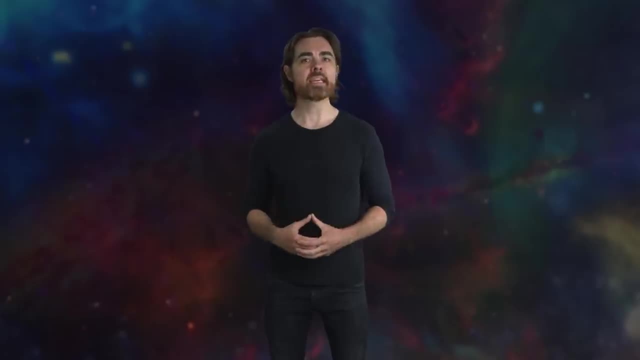 Or at the instant of the Big Bang. For that you need a true quantum theory of gravity. But even thinking about the structure of curved space on the smaller scales leads to craziness and catastrophic conflicts. I want to talk about these in two ways. 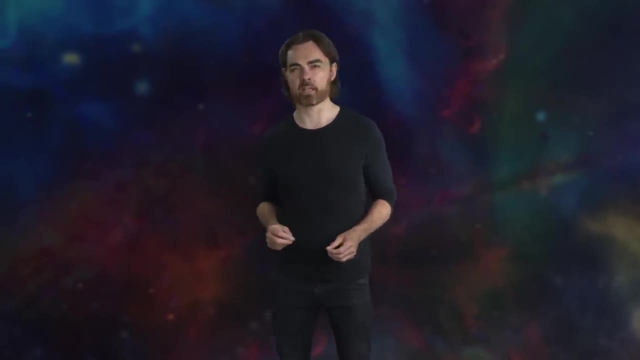 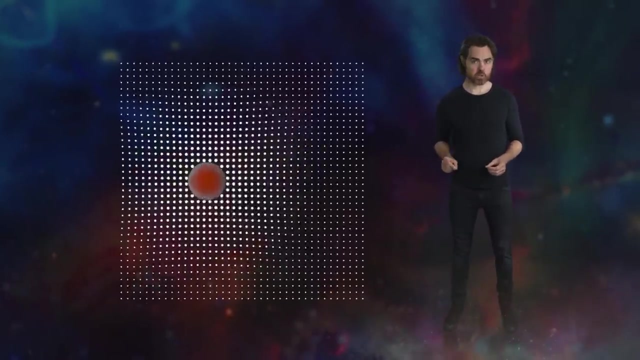 First very conceptually, Then a bit more technically. Let's start by thinking about what it means to define a location in a gravitational field with perfect precision, Or in other words, what it means to talk about very, very tiny chunks in the fabric of space. 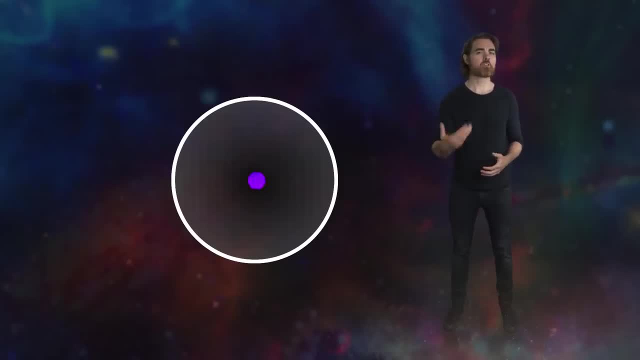 In order to measure a location in space, say the location of a particle, you need to interact with it. You would typically do that by bouncing a photon or other particle off the object. The more precisely you want to measure position, the higher the energy of that interaction. 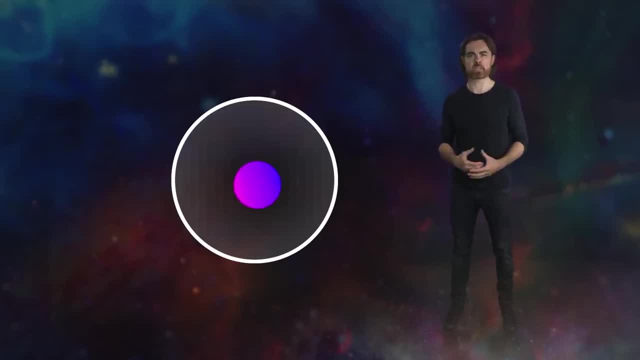 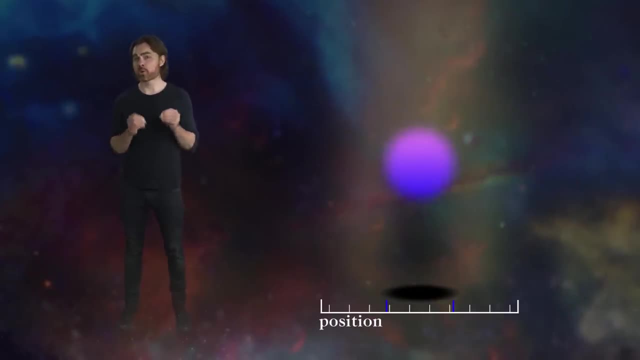 That's why we use electron microscopes or X-rays or even gamma rays to take images of extremely small things. So let's say we shoot a particle with a beam from a particle accelerator. We want to measure its location with extreme precision. The Heisenberg uncertainty principle. 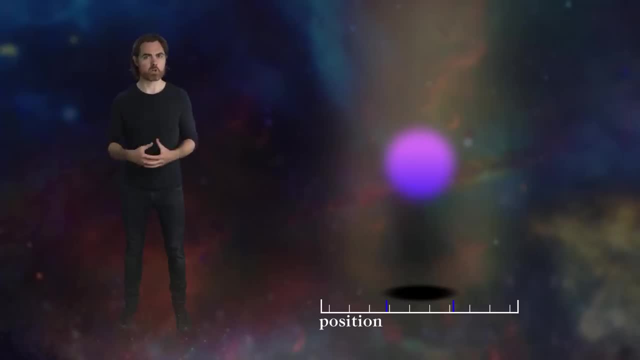 tells us the minimum energy of our beam for a given precision. It turns out that to measure a position to an accuracy better than a plunk length around 10, to the power of negative 35 of a meter, the amount of energy you would need to put into that region of space. 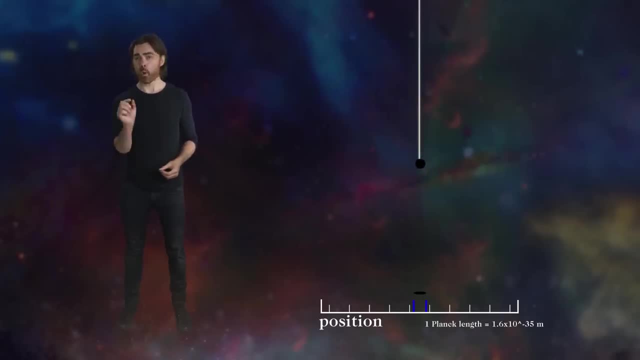 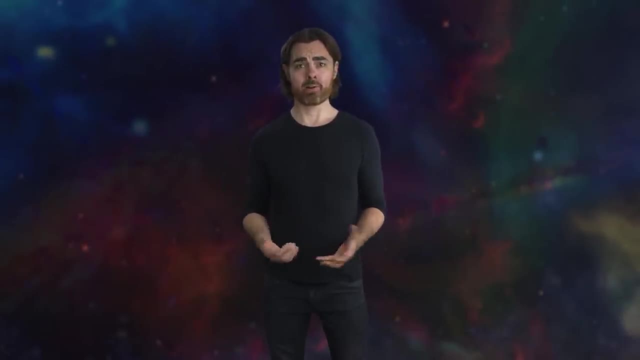 would make a tiny black hole with an event horizon one plunk length in diameter. Try to measure more precisely and you will need more energy. That means you make an even larger black hole. So general relativity plus Heisenberg say it's impossible to measure length smaller. 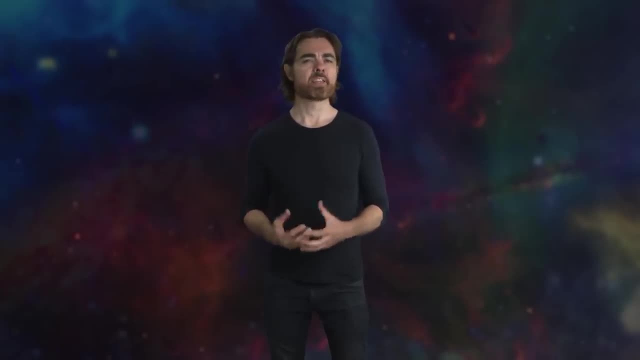 than the plunk length. Savvy viewers will remember that the uncertainty principle talks about the trade-off between position and momentum, But large momentum also means large energy. The uncertainty principle also defines the precision trade-off between time and energy, So this same argument can be used. 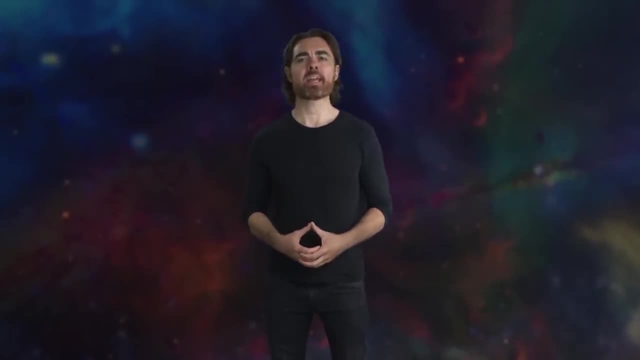 to suggest a fragmentation of time. Try to measure any time period shorter than 10 to the power of negative 43 seconds, the Planck time and boom black hole. For those of you who already watched our episode on the Heisenberg uncertainty principle, 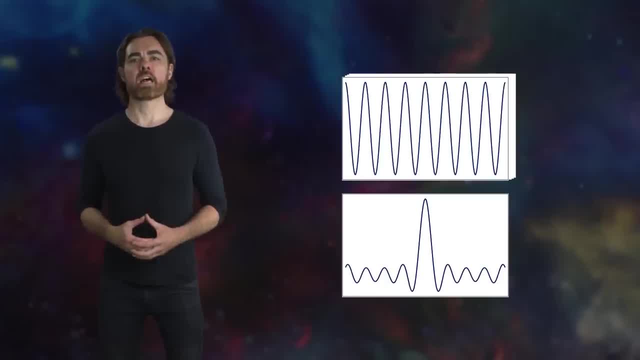 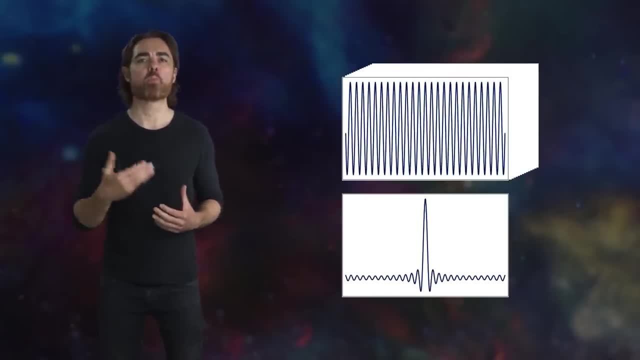 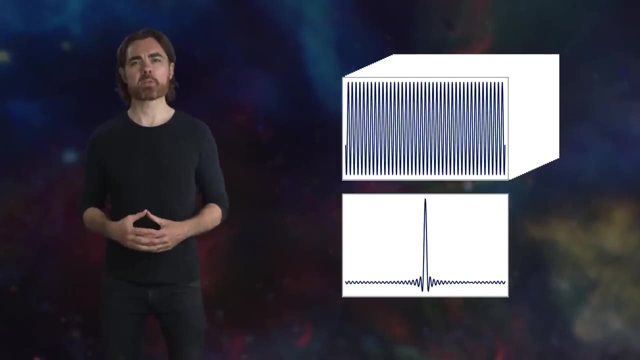 here's another way to think about this. We know that for a particle to have a highly defined location, its position wave function needs to be constructed from a wide range of momentum wave functions that include extremely high frequencies or extremely high momenta, ie the more certain its position. 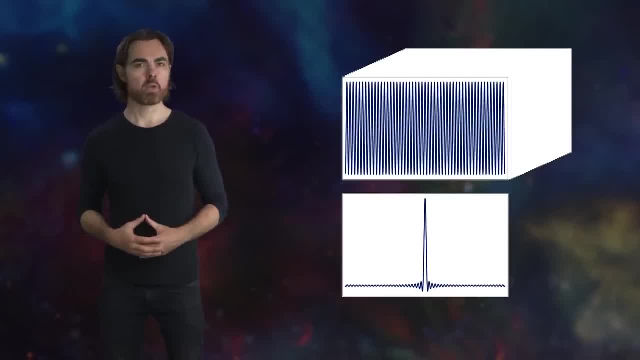 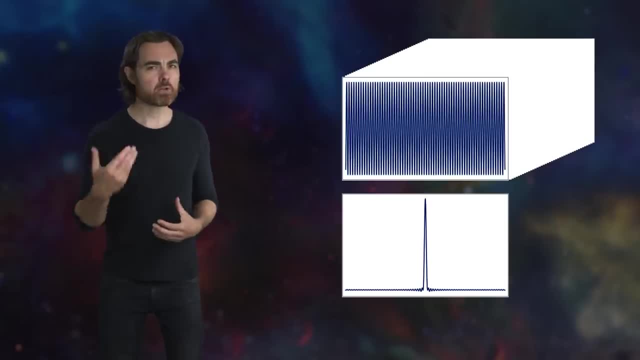 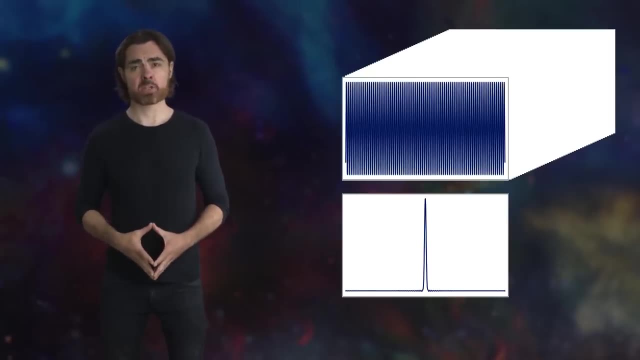 the less certain its momentum and so large momenta are possible. So position can be defined to within a Planck length and then momentum becomes extremely uncertain and includes the possibility of ridiculously high values. That means ridiculously high kinetic energies, particles whose positions are defined to within a Planck. 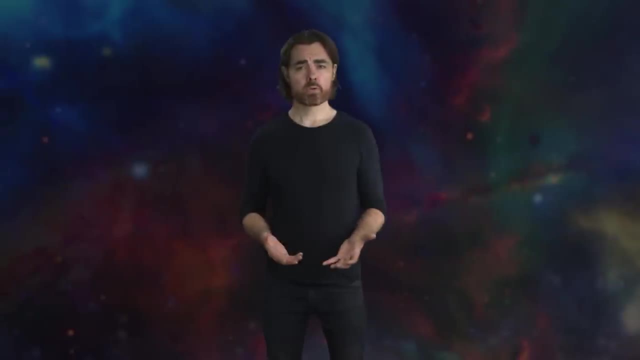 length can spontaneously become black holes. Of course, those black holes don't really happen. Rather, they're an absurdity that tells us that something is missing in our description of either quantum theory or general relativity, or both at the smallest scales. Let's look at the real conflict. Standard quantum theories treat the fabric of spacetime as the underlying arena on which all the weird quantum stuff happens. Given that sensible underlying structure, it's relatively routine to apply quantum principles or quantize most of the forces of nature. 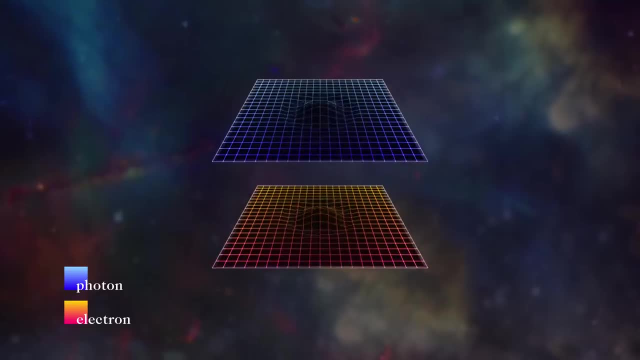 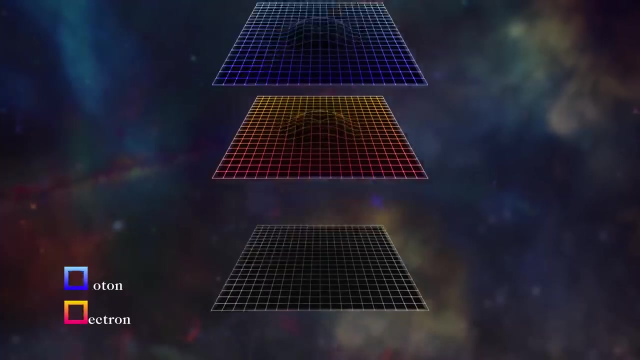 For example, classical electromagnetism becomes quantum electrodynamics when you quantize the electron field and the electromagnetic field. But in the resulting math the new quantum fields still lie on top of a smooth, continuous grid of space and time. So what if you want to quantize gravity? 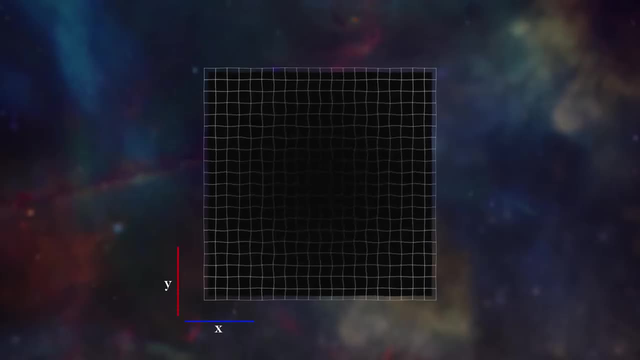 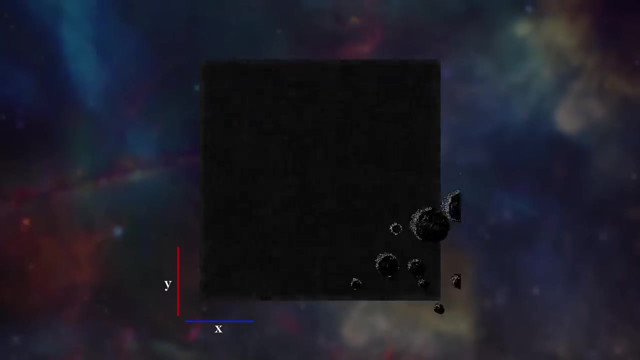 The gravitational field doesn't lie on top of spacetime, It is spacetime. To quantize gravity, you have to quantize spacetime itself. That leaves no clean coordinate system on which to ground your theory. This sounds annoying. In fact, it's a disaster. 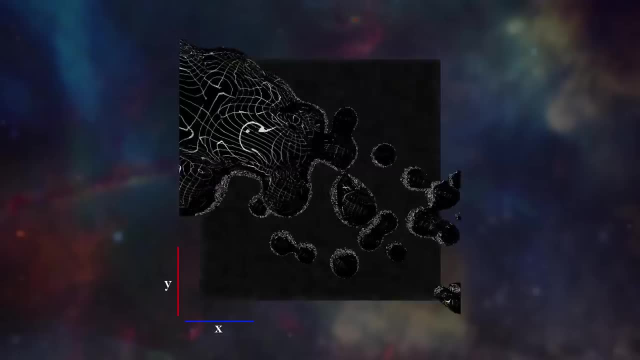 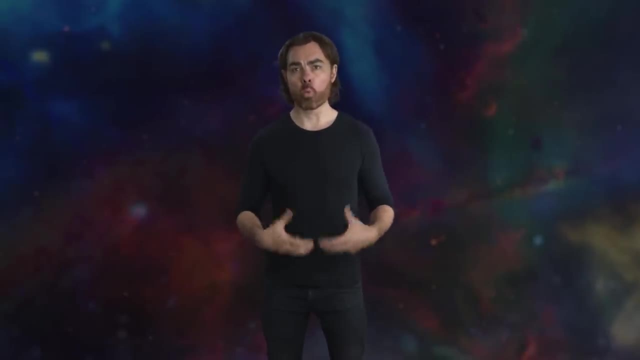 It leads to several problems, But I'll focus on the one that wrongly predicts these crazy fluctuations on the Planck scale. In general relativity, the presence of mass or energy warps the gravitational field. There can be no exceptions. Any energy must cause spacetime curvature. If not, you could build perpetual motion machines, for example using the Casimir effect. In quantum gravity, gravity itself becomes an excitation in our quantized spacetime. The energy of those excitations should themselves precipitate more spacetime curvature. 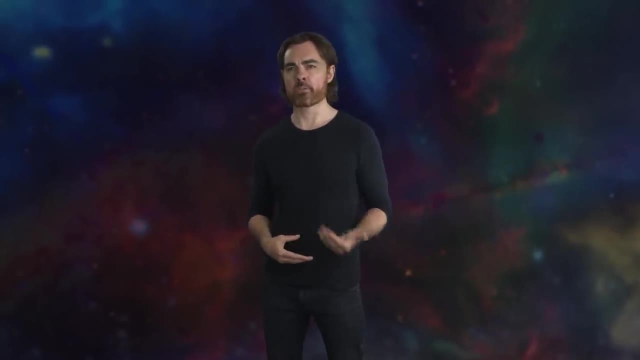 represented as further excitations. In other words, gravity should produce more gravity ad infinitum. This type of self-interaction or self-energy is seen in other quantum field theories and is hard to deal with even there, For example in quantum electrodynamics. 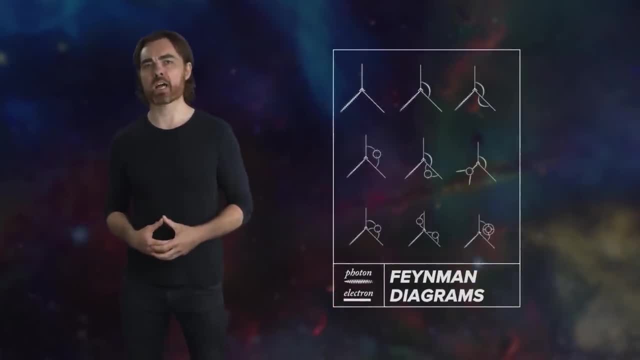 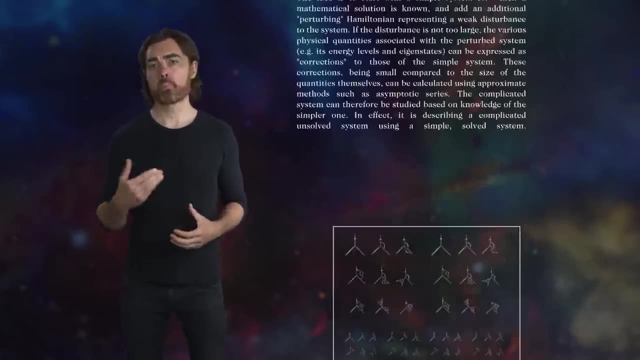 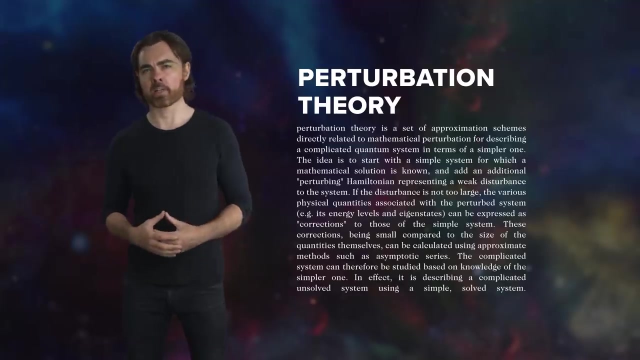 the electron has a self-interaction due to its electric charge messing with the surrounding electromagnetic field. In QED the mess is fixed with something called perturbation theory. It's a scheme to calculate a complex interaction like the buzzing electromagnetic field around an electron. 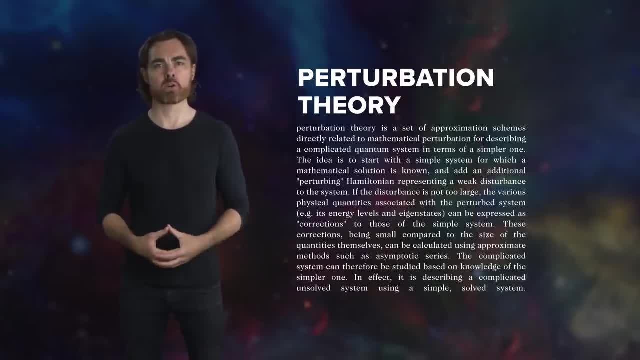 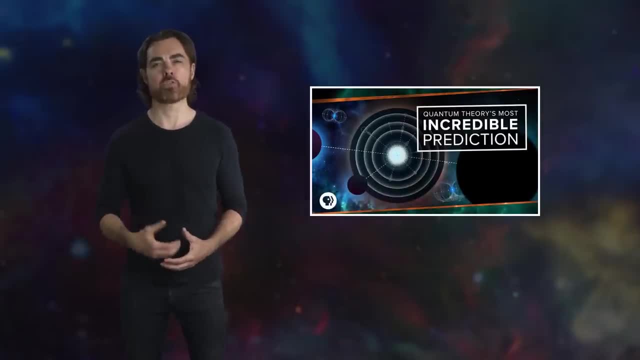 with a series of corrections to a simple, well-understood interaction which might be the electron in a quiet electromagnetic field. We talk about this more in our episode on the g-factor. So perturbation theory is applied throughout quantum field theories of the standard model. 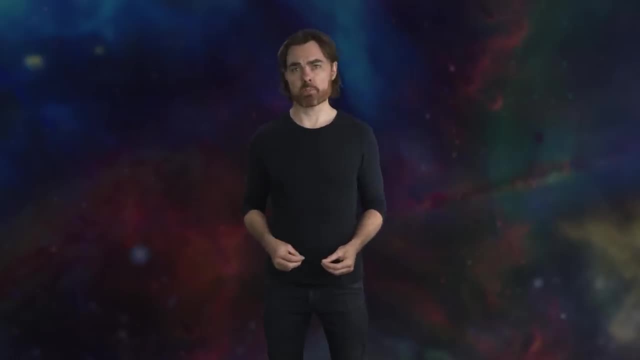 and it works because, one, these corrections are small And or two, even in the case where the corrections appear large or even infinite, they can be constrained, They can be brought back to reality by actual physical measurements of a few simple numbers. 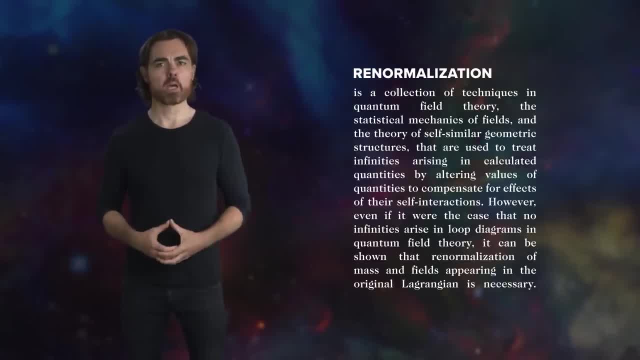 in a process called renormalization. For example, measurement of the mass and charge of an electron renormalizes quantum electrodynamics to allow incredibly precise calculation of the electron's self-energy. None of this works when you try to quantize general relativity. 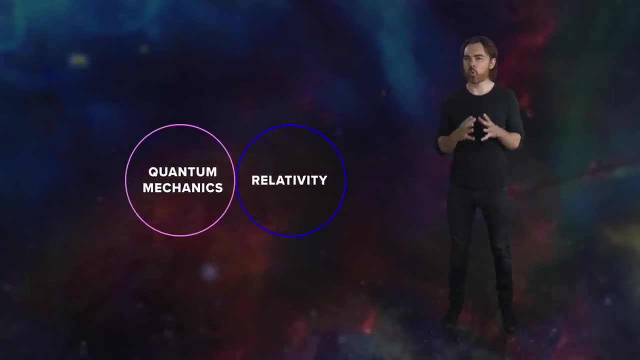 When you have strong gravitational effects on the quantum scale, the self-energy corrections blow up to infinity. But unlike other quantum field theories, there are no simple measurements you can do to renormalize those corrections. In fact you would need infinite measurements to do so. 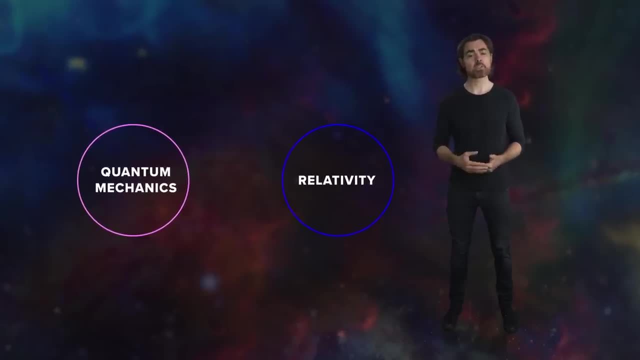 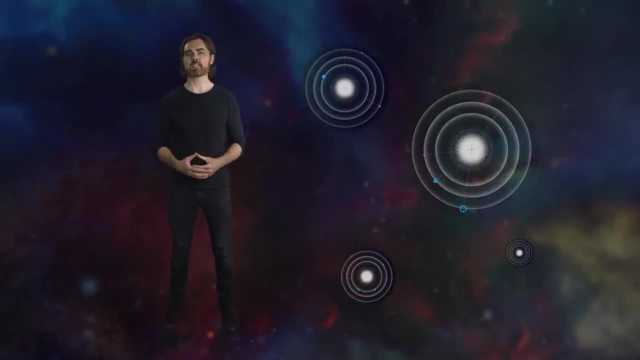 We say that a quantized spacetime of general relativity is non-renormalizable. The non-renormalizability of quantized general relativity is connected to the idea that precisely general relativity, precisely localized particles, produce black holes. 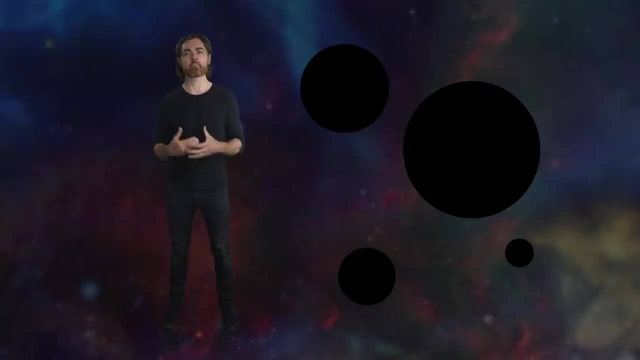 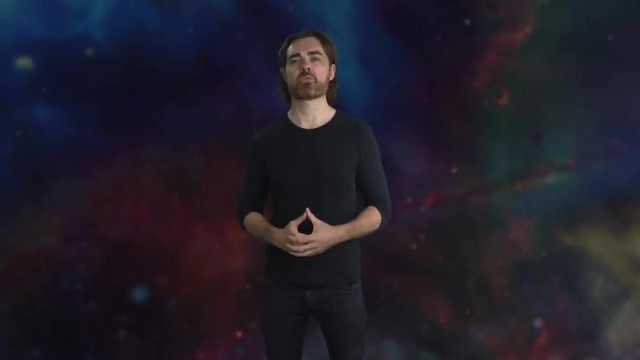 Space and time simply cannot behave in the familiar way below the Planck scale, And so the simplest approach to quantizing gravity and spacetime must be wrong. Generations of physicists, starting with Einstein himself, spent their lives trying to fix this, to unite quantum mechanics and general relativity. 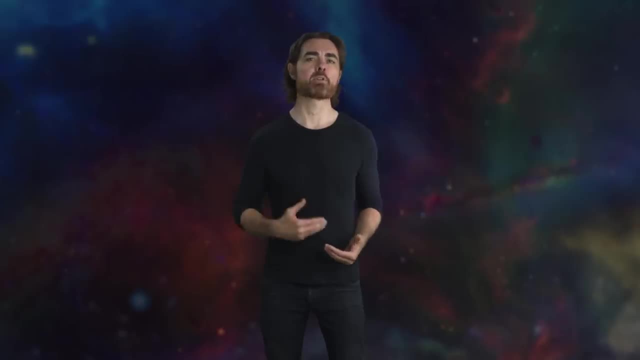 They are still trying, Even though we still lack an accepted resolution. the struggle has not been without progress. There are two main approaches. One is that you search for a way to quantize general relativity in a way that avoids the infinities. 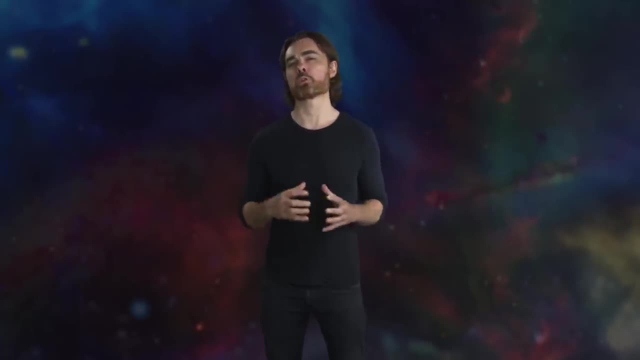 and non-renormalizability. The leading example of this is loop quantum gravity. Or you just assume that GR, and indeed the mutable fabric of spacetime itself, are emergent phenomena from a quantum theory deeper than our currently accepted theories. That's exactly what string theory seeks to do. 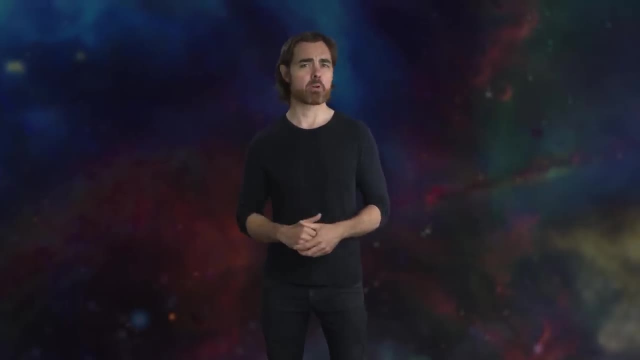 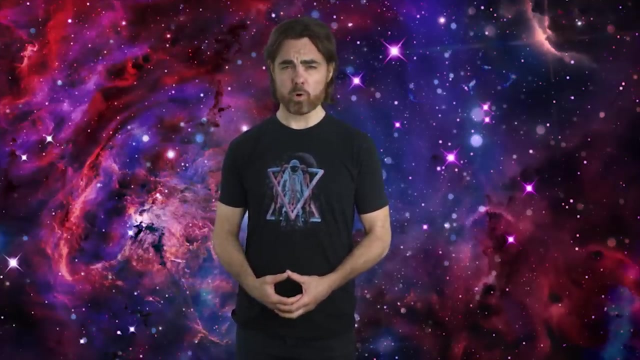 In upcoming episodes we'll explore these and other ingenious approaches to crack the greatest problem in modern physics: the quest for a theory of quantum spacetime. Hey everyone, So we haven't done a Patreon shout out in a while. Why? Because the Patreon crew already hangs out with us. 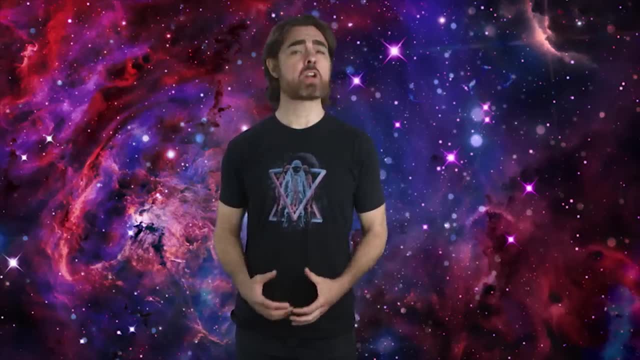 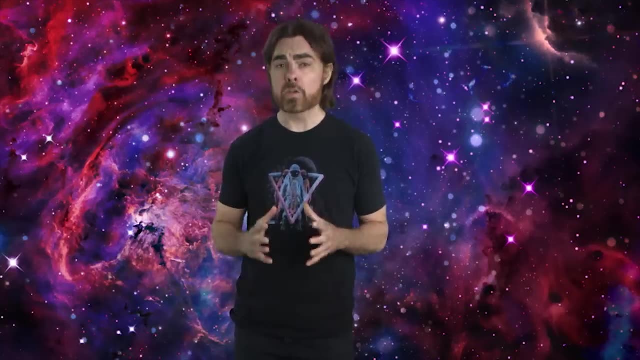 on Google Hangouts and on the content selection team and in general, on the Patreon site. Want to hang out with us, Please? We would love to have you, But I digress. Thank you so much, Patreon supporters. You make all of this possible. 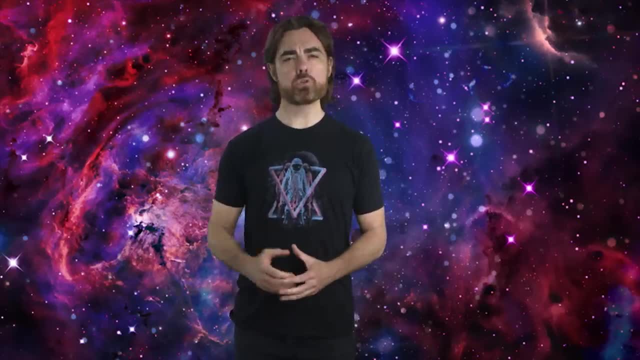 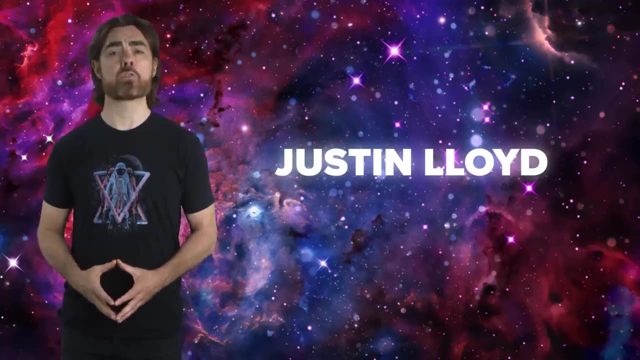 All of this much easier for us, And today a special, huge thank you to Justin Lloyd, who's contributing at the quasar level. Justin, as a special thanks, we're sending you a box of chocolate-covered Planck scale black holes. 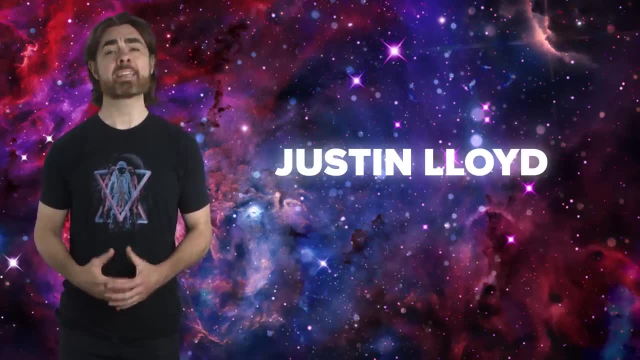 If our modern understanding of Hawking radiation is right, they will evaporate catastrophically long before they reach you. Let us know if you get them. It'll really help us constrain some black hole theory. OK, so on to comment responses. 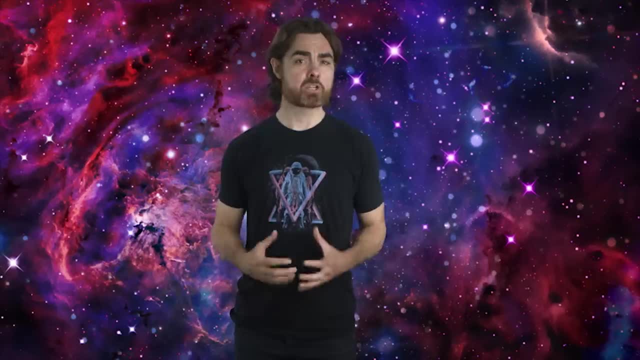 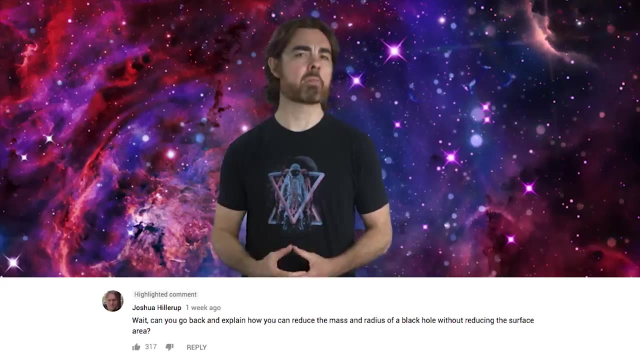 Today we're covering both the black hole entropy enigma and the challenge question episode: how much information does the universe contain? A few of you asked why it is that the surface area of a black hole's event horizon must always increase and how mass and radius can actually decrease. 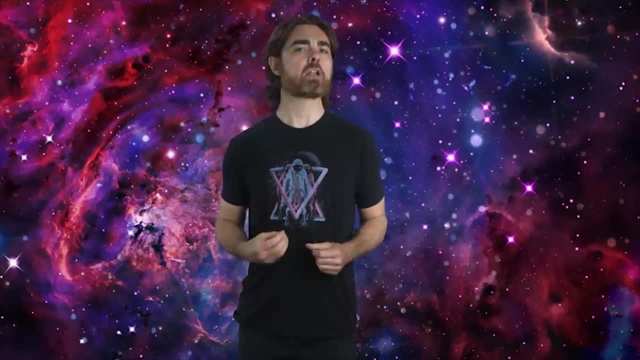 Well, let's talk about the latter. When two black holes merge, a lot of energy is pumped into gravitational waves. There's only one place for that energy to come from: the mass of the black holes. As a result, the mass of the final merged black hole. 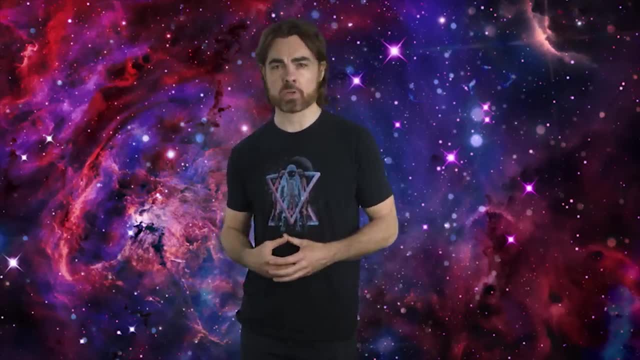 is smaller than the sum of the mass of black holes, That's the sum of the masses of the two originals. Event horizon radius is proportional to mass, and so the radius of the final black hole is smaller than the sum of the radii of the originals. Note that the final black hole is both more massive and larger than either of the original black holes taken separately. Then there's the Penrose process. It's possible to extract energy from a rotating black hole by throwing in objects on near-miss trajectories. 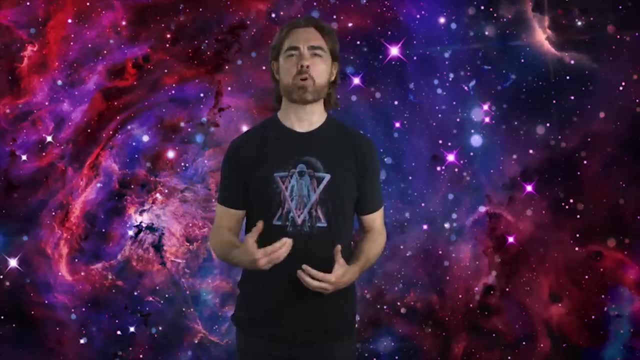 The rotating black hole drags space around with it and the incoming object of the black hole, which absorbs some of that rotational energy and gets flung out at a higher speed. The loss of rotational energy by the black hole also means a loss of mass. 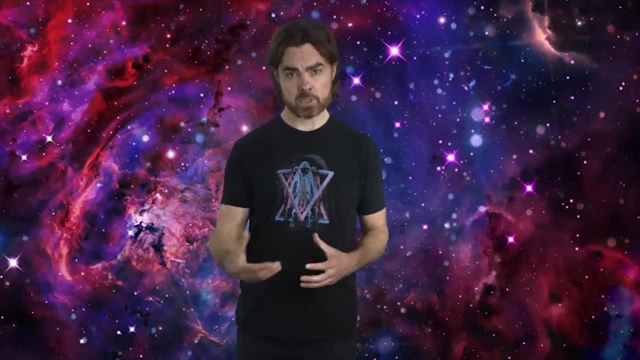 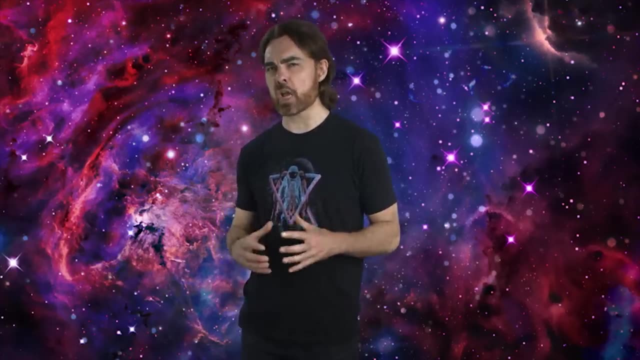 But rotating black holes are slightly squished As they lose spin. angular momentum, they become more spherical. In that process the event horizon only changes shape, It doesn't lose surface area. Debeste points out that it's important to emphasize. 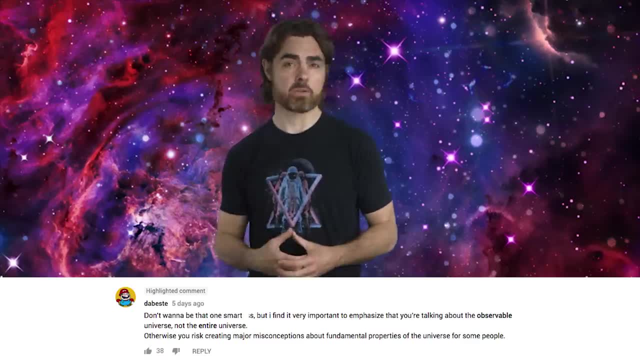 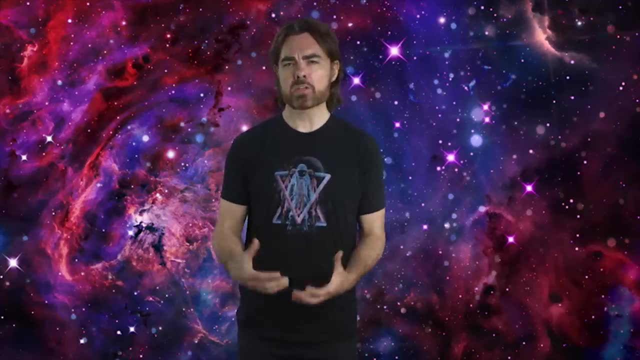 that you're talking about the observable universe, not the entire universe, And I totally agree. For those of you who had doubts, the challenge question is asking for the size of the storage device needed to store all of the information in the observable universe. 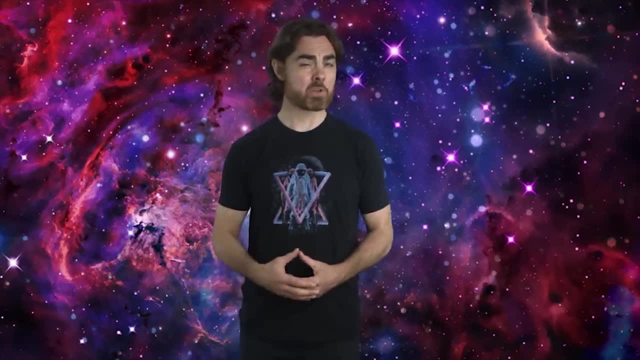 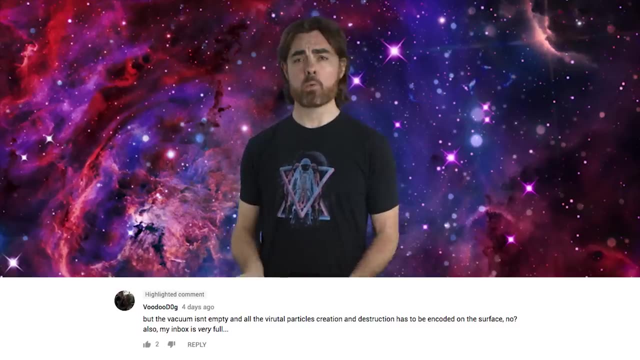 I said observable near the start of the episode, but I dropped that observable part a couple of times later on. That's my bad. Voodoo Dog points out that the vacuum isn't really empty what with all the virtual particles popping into and out of existence. 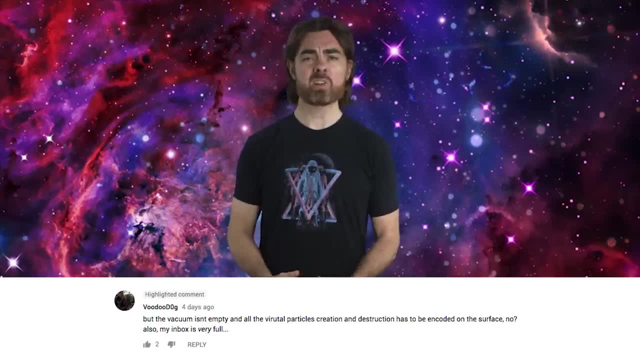 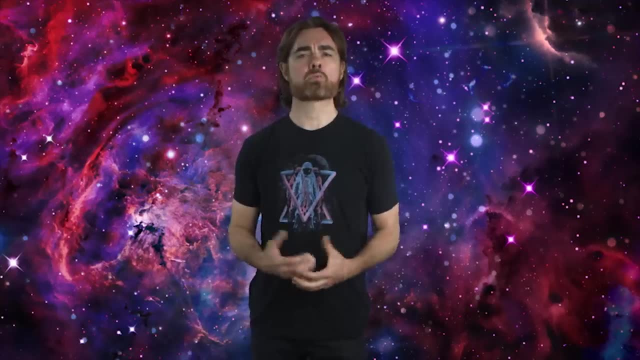 So what about their information? Well, actually, those don't really contain information, because they aren't real In the sense that we think of normal particles. The phantom, virtual particles represent both the absence of particles and every possibility of particles, But in both cases there's no specific defined state.